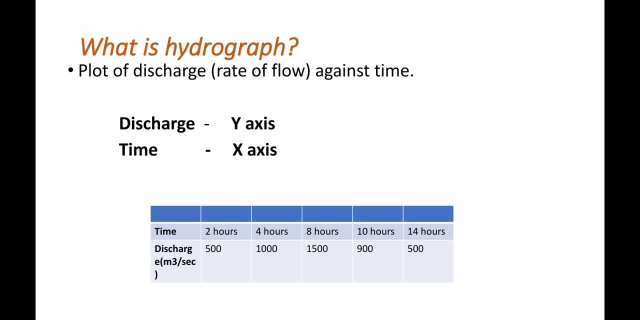 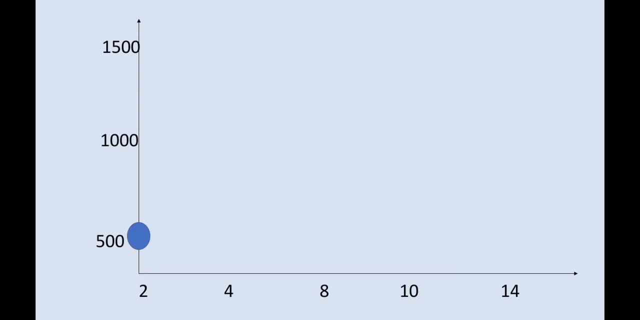 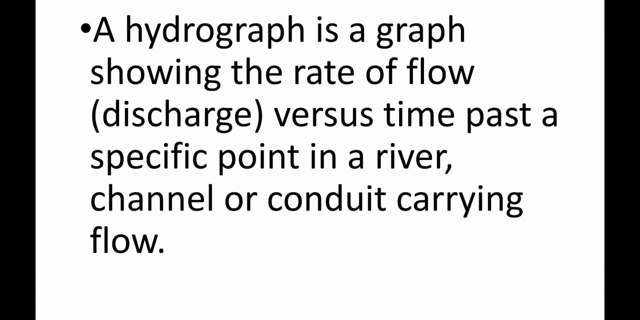 At 10 hours it is 900 m3 per second And at 14 hours it is again 500 m3 per second. We plot this part on the graph and this graph is called hydrograph. Now look at the second definition, What it is saying. 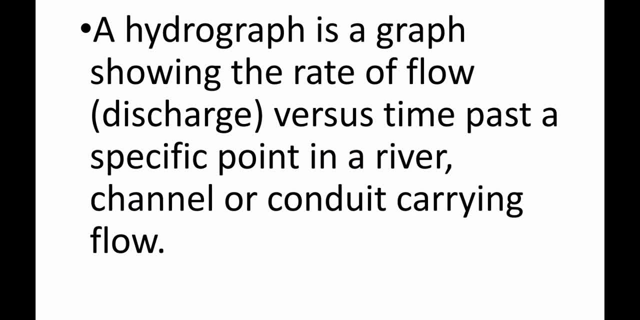 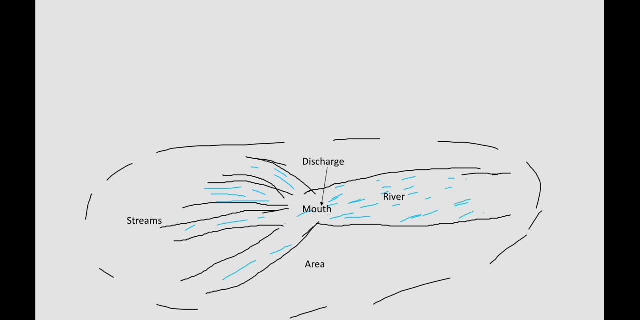 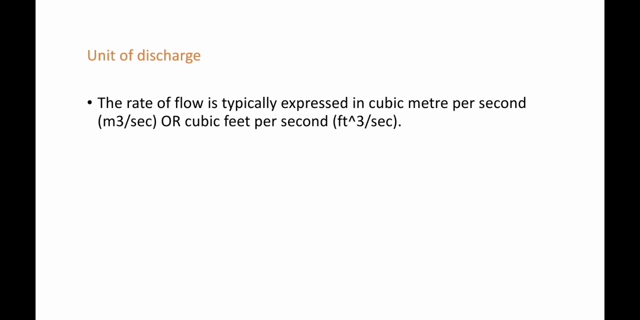 want to know the discharge or amount of water which flow at the mouth of the river at different time through this area after starting of rainfall. we can use hydrograph for that. we typically express discharge or we can say rate of flow in cubic meter per second or cubic feet per second and time in hours. 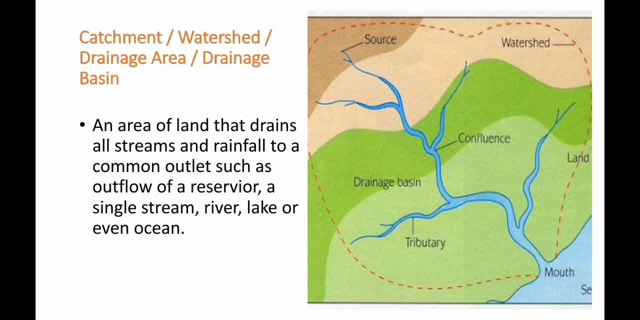 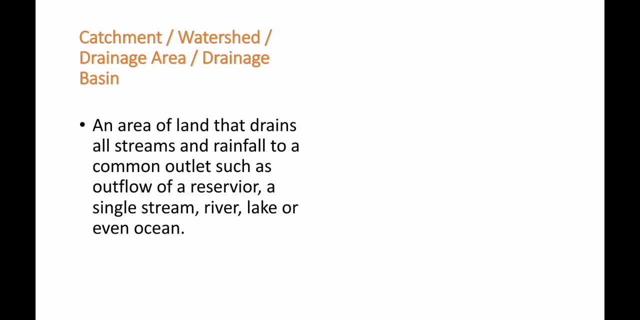 let us understand what is catchment, watershed or drainage area or basin area that we will see how it is going to be used in the future, how our hydrograph look like: an area of land that drains all streams and rainfall to a common outlet such as outflow of reservoir, a single stream. 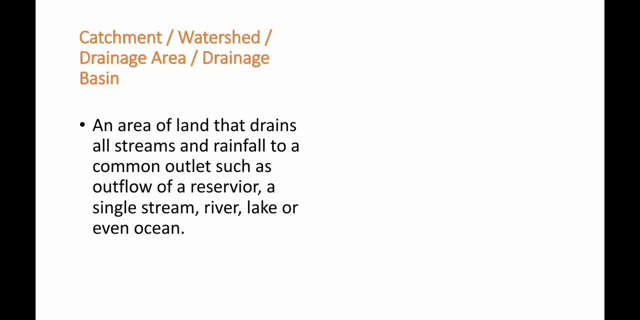 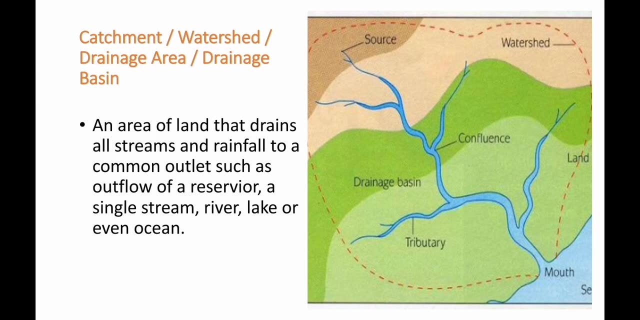 river, lake or even oceans. it means a catchment is the area from which all the water from the stream and rainfall goes to a common outlet. look at the image shown. the area surrounded by the dotted line is a catchment, or we can say watershed or drainage area. you can see all the water streams in this area are drainage their. 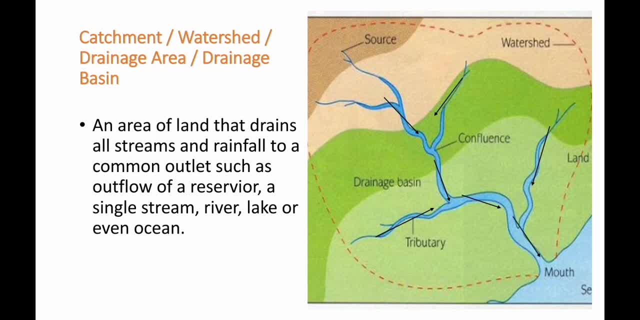 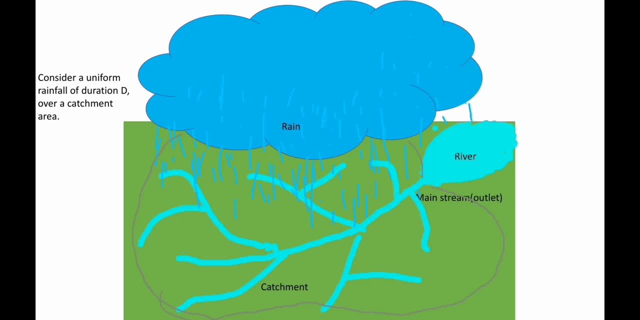 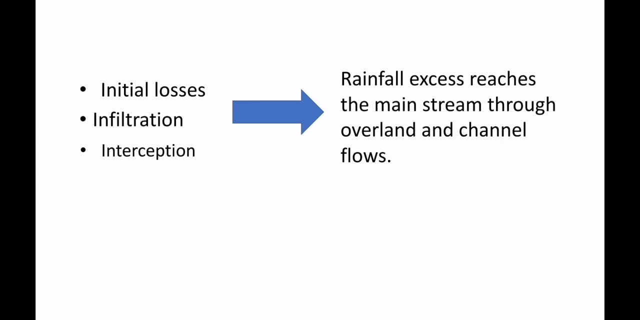 water to a common outlet at mouth of sea. suppose this is a catchment area and rainfall for duration d occurred over this area. what will happen initially? there will be loss due to process like infiltration, interception etc. and the water will take time reach the outlet. there will be lacked time between start. 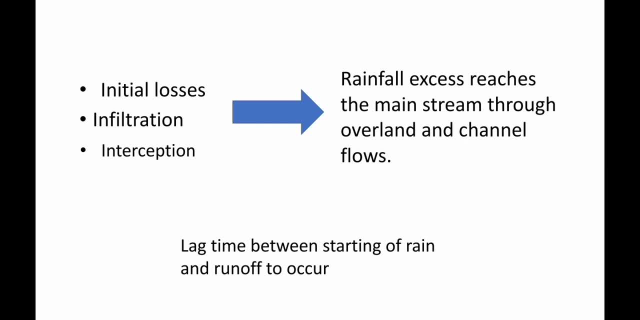 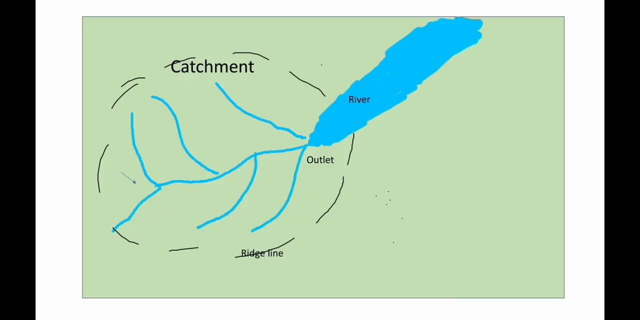 of rain and run off or discharge to occur. so initially the discharge will not increase. after some time, when soil will be saturated. after this loss, the water will collected over the land and will reach the streams, and the streams will discharge water at the outlet or at the mouth of river. thus discharge at 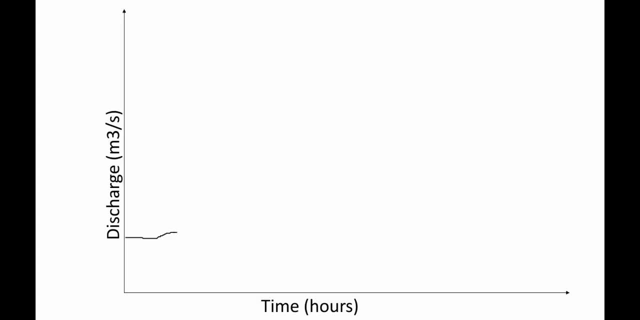 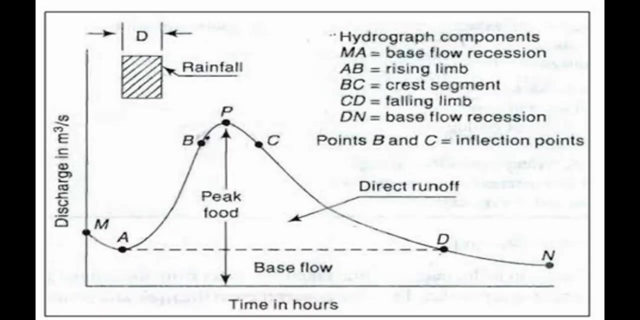 outlet will begin to increase and after some time will attain a maximum amount of discharge and then it will begin to decrease and will decrease further after rainfall will stop and will again reach the point of initial groundwater flow. so our graph will be something like this. you can see a clear picture of the graph. 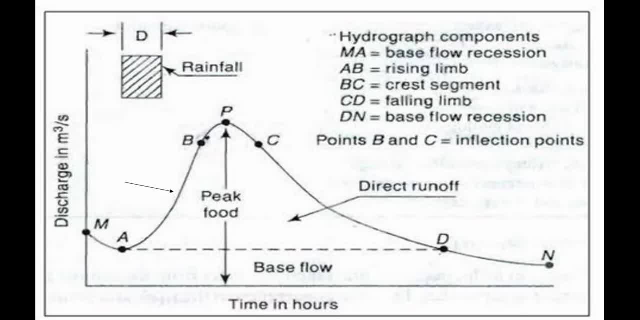 this part of a graph, a to B, in which runoff or discharge is increasing is known as rising limb, and this is the crest segment from B to C in which peak flow occurs, highest amount of flow occurs. this is falling limb, or limb from C to D, in which the 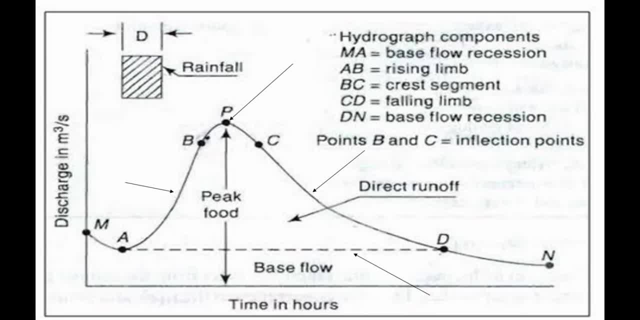 flow rate decrease. this section from A to D is called base flow, means groundwater flow, which was initially there, and the above portion, which surface runoff occurred, is called direct runoff. this is the rainfall data shown which tells the duration D and rainfall depth. we will learn in detail. 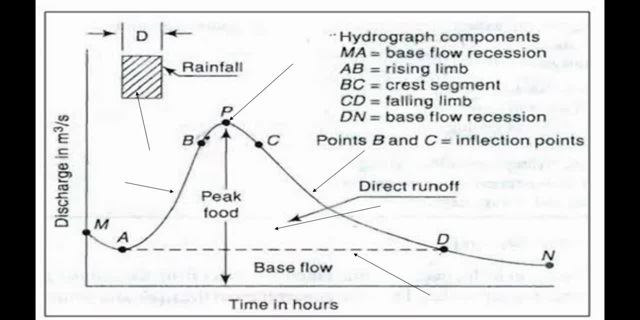 about component of hydrograph in next video lecture. so please like and subscribe our channel for more updates. thank you. 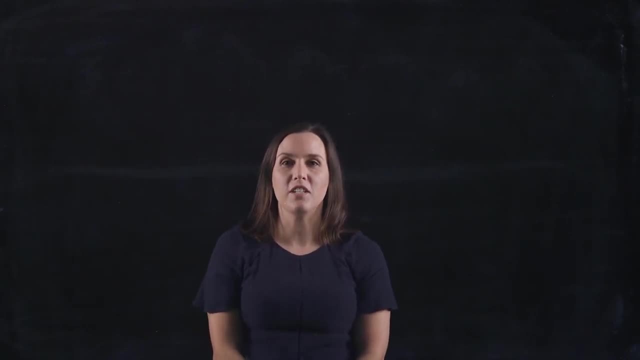 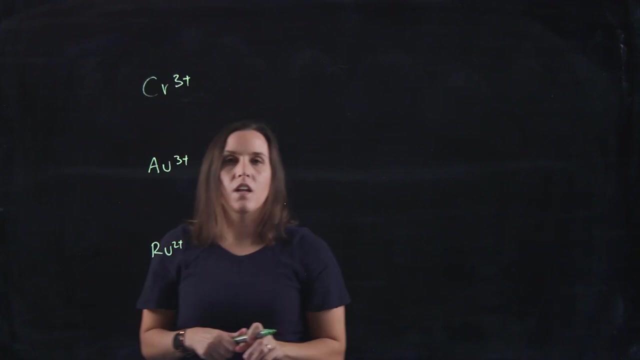 Hi, so welcome to another video. So in this video we're going to be looking at the electronic configuration of some of the transition metals. So let's look at these three first. So we've got Cr3+, Au3+ and Ru2+. 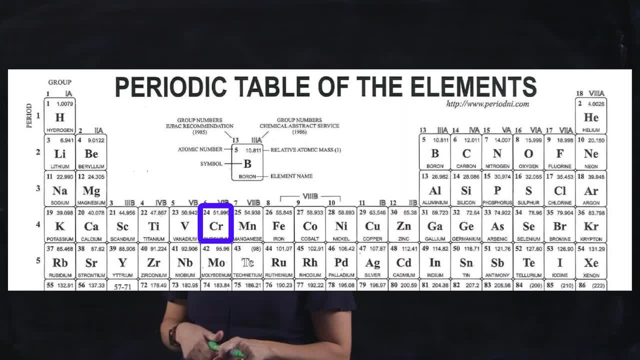 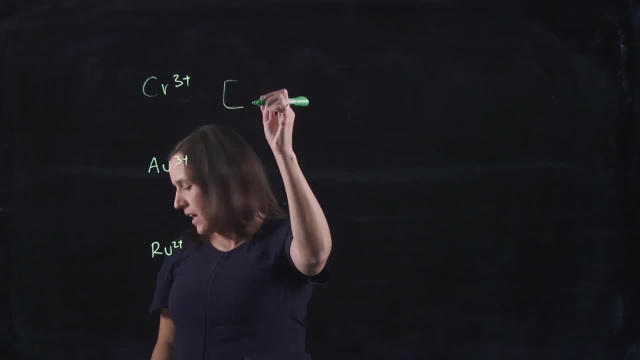 So, first of all, finding where Cr is on your periodic table, So you can see that your periodic table has the Cr, so the chromium, which is element number 24.. So it's a. if I write the abbreviated one, so I go across to argon, everything is. 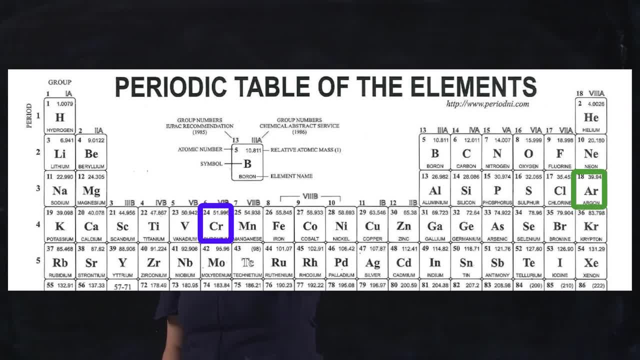 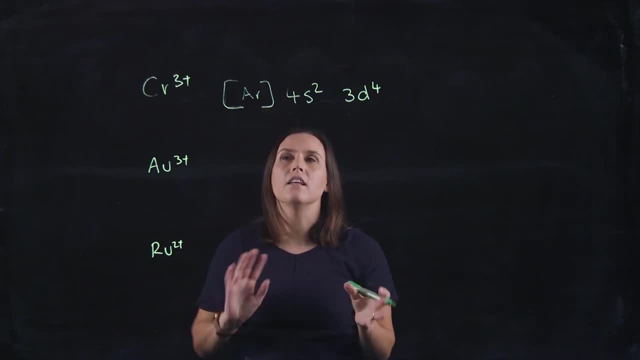 the same up until argon, and then the difference is your 4s2, and then we've got 1, 2, 3, 4, 3d4.. So, with our transition metals, when we're looking at the 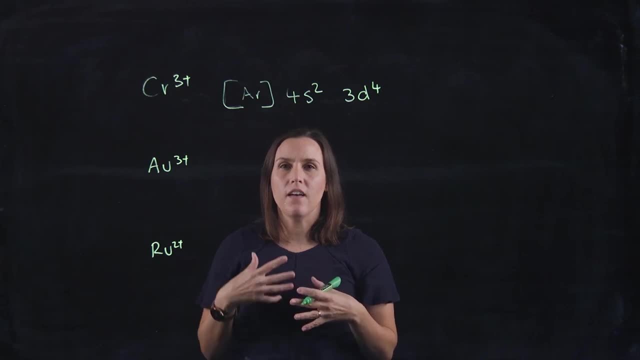 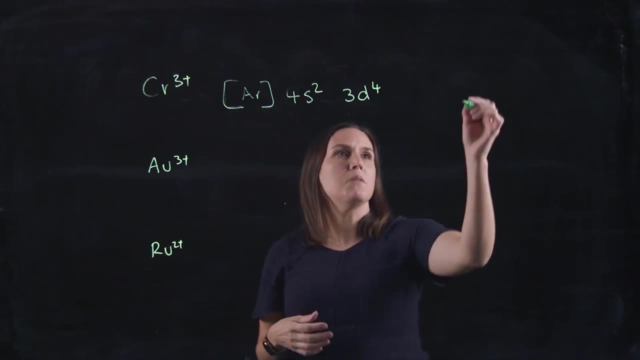 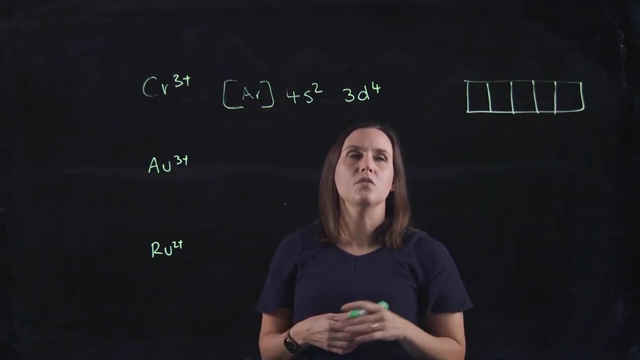 electronic configuration. remember there's an electronic configuration. remember there's an advantage to half filling those d orbitals and completely filling because they drop down in energy. So remember your d block has 5, 1,, 2,, 3,, 4, 5 orbitals.